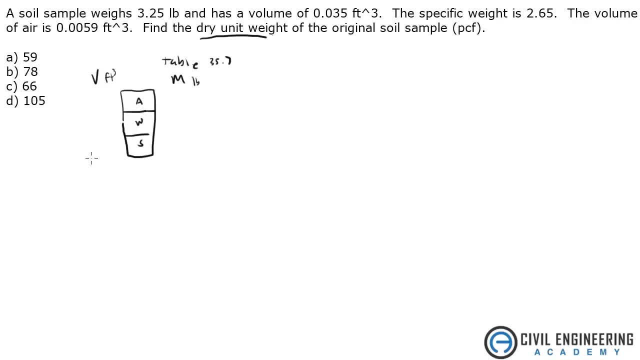 And that's in cubic feet and this is in pounds And you can total these up. Air was given as 0.0059.. Mass of air is 0.. The mass total was 3.25 pounds and the volume was 0.035.. 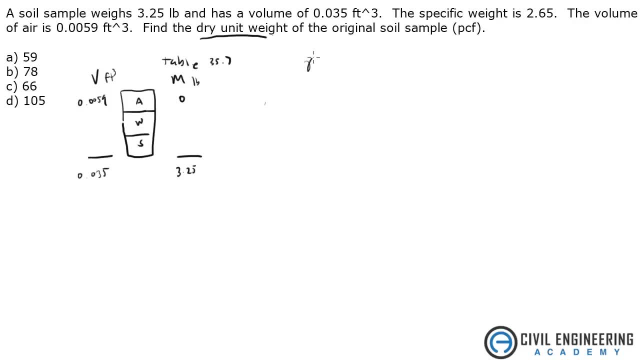 So we were given this. We also know from this table that the dry density is the mass Of the soil divided by the total volume. So those are the things we need to find. We know the total volume, but we do not have massive solids. 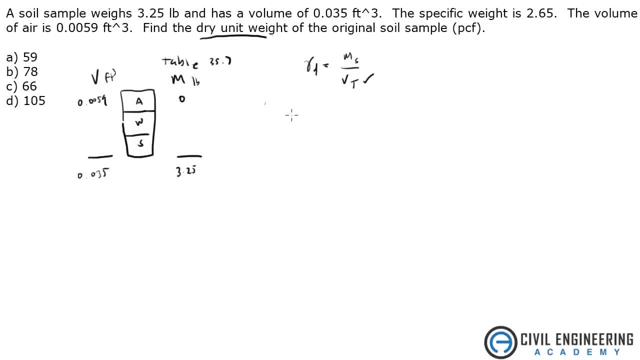 So the first thing I'm going to recognize is that the volume of water plus the volume of the soil is equal to the total 0.035. subtract out the air, 0.0059.. And that gives me 0.029.. So if we know that, if we can solve for the volume of the soil, 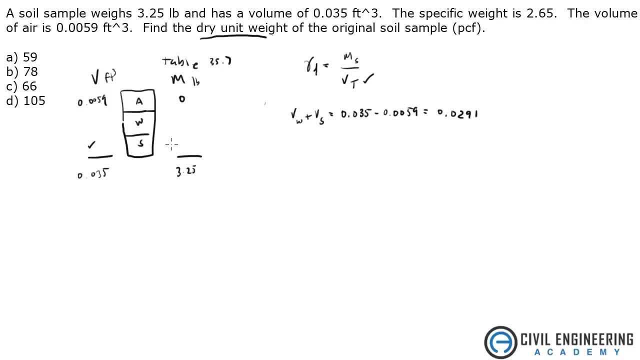 then I believe we can probably get the mass of the soil Which is all we need to get this thing done. So we know this equation. This is a good equation. Let's try to get another one. Well, we know specific gravity That was given to us. 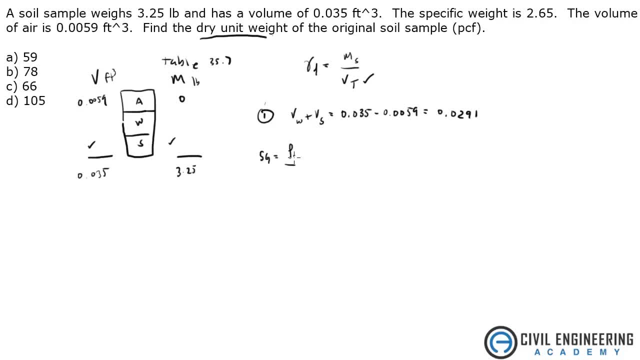 We know that's basically the density of whatever you're solving for, In this case the soil divided by the density of water. Or it could be rewritten as the mass of the soil over the volume divided by the density of water. And if I go ahead and rewrite all of this, 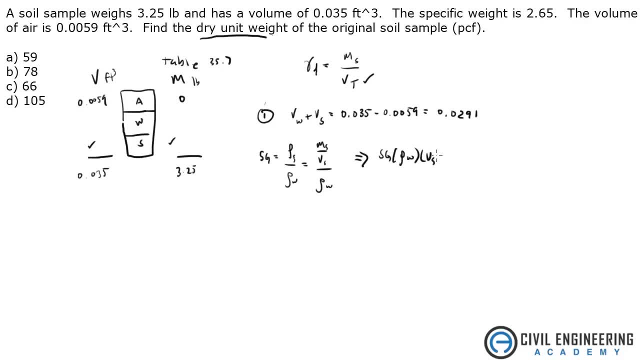 I can get specific gravity times. density of water times the volume of the soil is equal to the mass of the soil. You also know that the density of water is the mass over the volume of water And if you rewrote that you could get density of water times the volume of water. 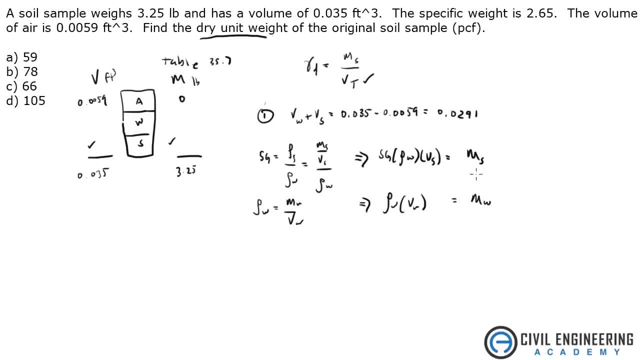 is equal to the mass of the water, And if you added those two things together, you would get the total mass which we know. So if we use this as an equation- and we already have one equation up here, We already got one there- 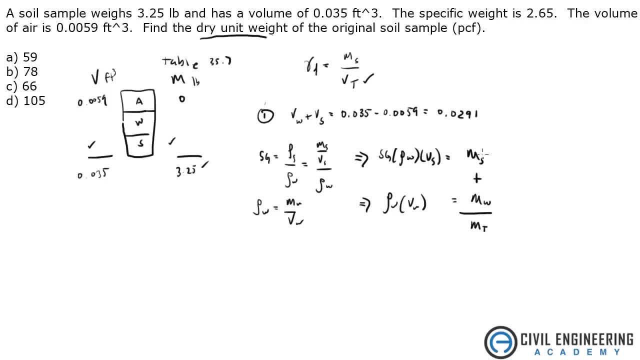 But yeah, you get the idea. If we have an equation here and we use this as another equation, then we can solve for one of these variables And let's go ahead and do that. So the mass of solids plus the mass of the water: 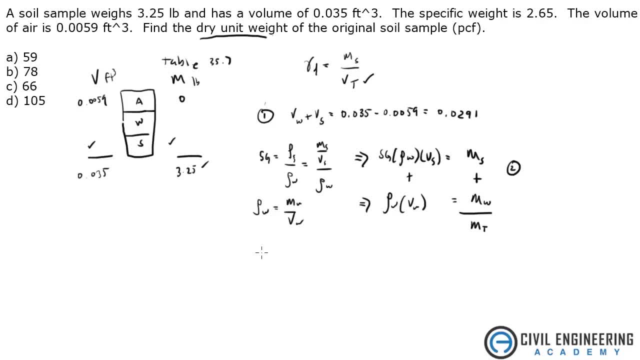 And I'm going to rewrite it with these two variables. Add these two things together, So the specific gravity is 2.65 times 62.4 pounds per cubic feet. density of water- times Vs- which we don't know- Plus 62.4 times Vw. 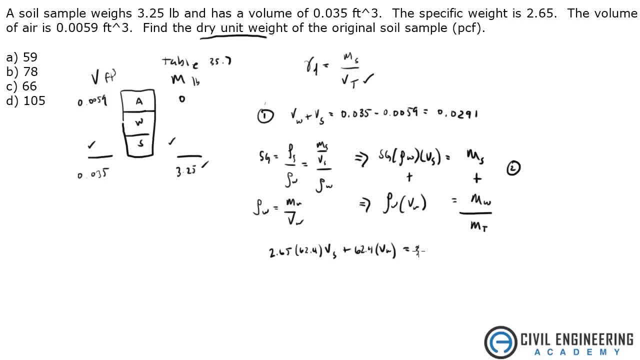 is equal to the total mass, 3.25.. Okay, Carry all those through and rewrite it. So that's 165.36 Vs plus 62.4 Vw is equal to 3.25.. So if I rewrite this equation up here, 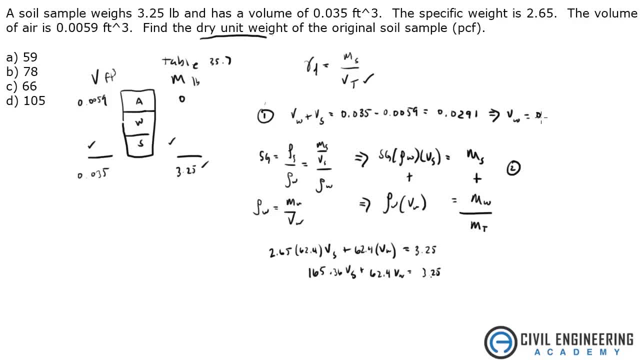 in terms of Vw: 0.0291 minus Vs. If I take that into this equation, plug it down there, I get a Vs equal to 0.014. when you plug all that in and solve for it, So that gives me the volume of the solids: 0.014. 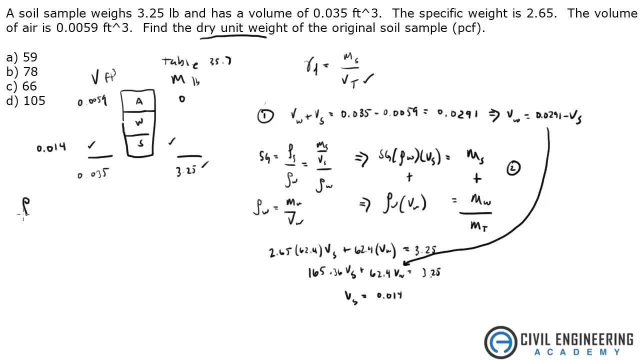 Now, how am I going to get the mass of the solid? Well, we know that the density of the solid or the soil- sorry, I keep saying solid- is the specific gravity times the density of water. We also know that the density is the mass over the volume. 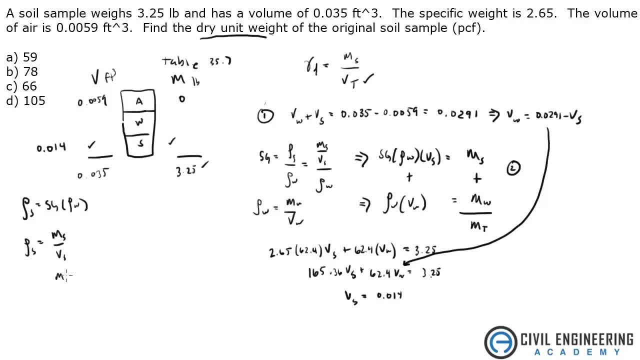 So if we just set those two equal to each other, mass over volume is equal to specific gravity times the density of water. Bring the volume to the other side and you get 2.65 times 62.4 times Vs, which we just solved for 0.014..